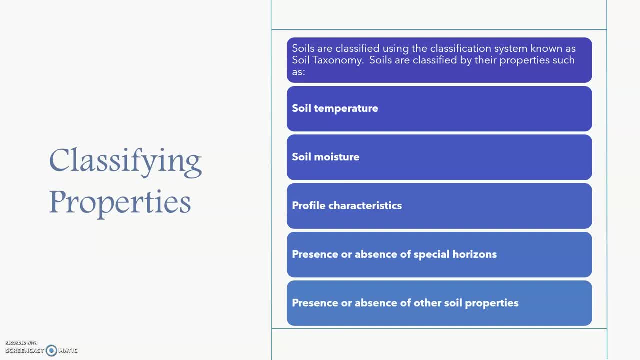 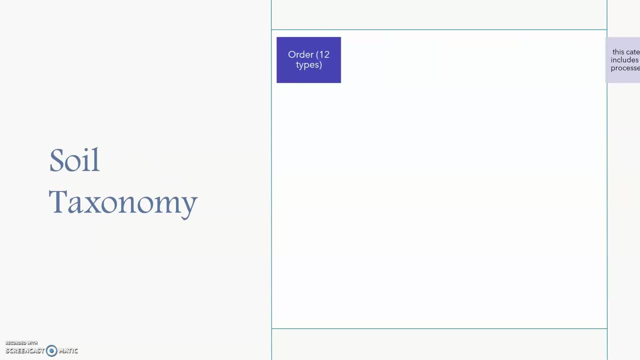 of special horizons and presence or absence of other soil properties. Soil taxonomy starts with soil orders. There are 12 soil orders. Soil orders are based on the soil forming process. Soil orders include soils with properties resulting from similar soil forming processes. A soil order is the most general category. Soil orders are divided into suborders. 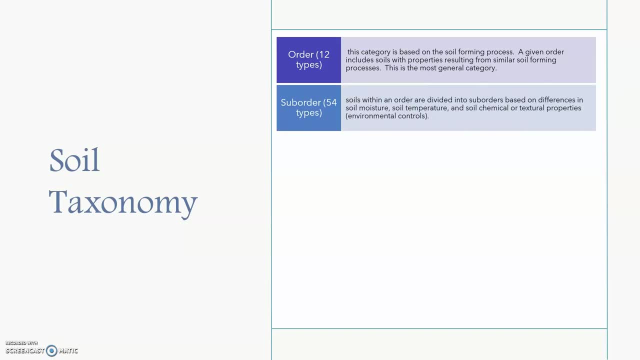 There are 54.. Suborders are divided based on differences in soil moisture, soil temperature and soil chemical or textural properties. Suborders are divided into grate groups. There are more than 240 of these. There are more than 240 of these. 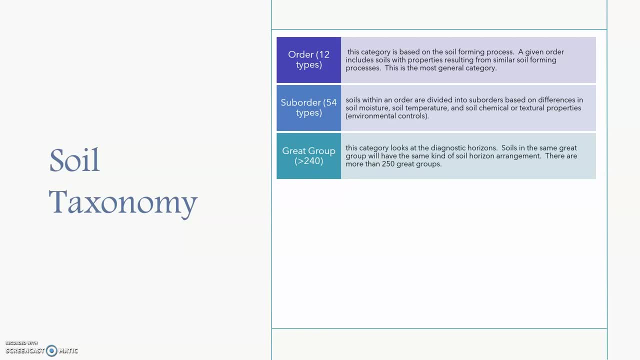 Grate groups look at diagnostic horizons. Soils in the same group have the same type of soil horizon arrangement. Grate groups are further divided into sub westerns. There are more than 1,300 subgroups. Subgroups are divided into types There. 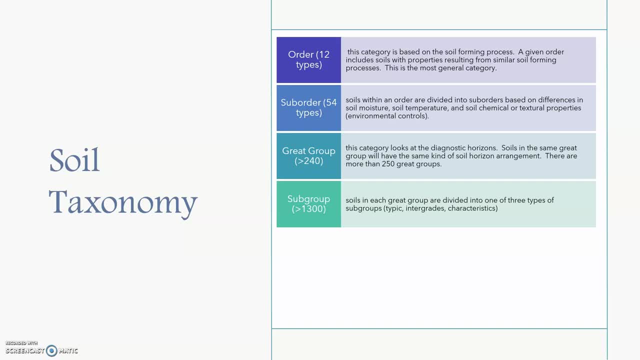 are three types: typic, integrates and characteristics. Subgroups are further divided into families. There are more than 8,000 soil families. Soil families are based on properties important for plants or engineering purposes. Lastly, families are divided into series. There are more than 23,000 soil series. 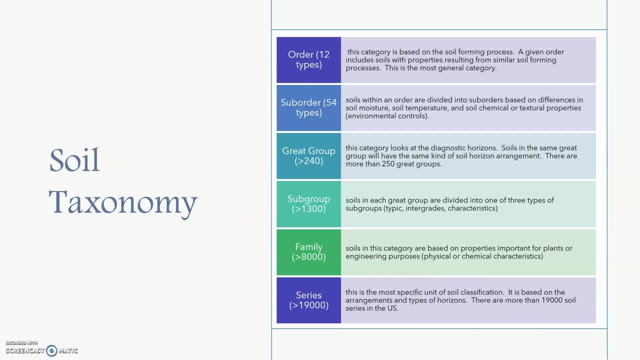 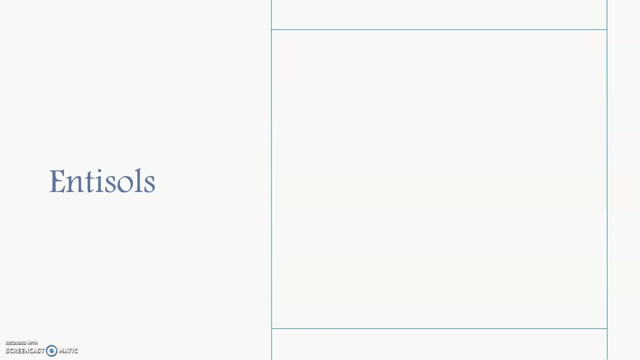 worldwide Soil series is the most specific unit of soil classification. It is based on the arrangements and types of horizons. There are more than 19,000 soil series in the United States alone. The first soil order we are going to look at are entosols. Entosols are soils. 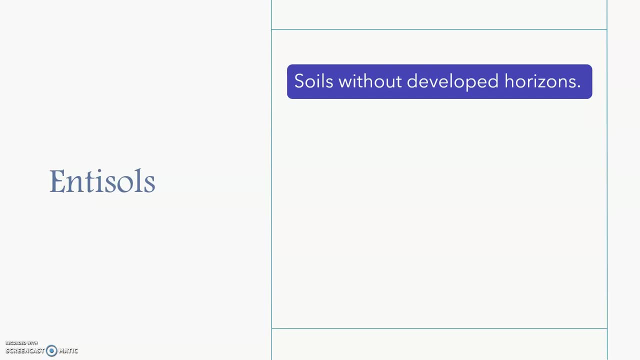 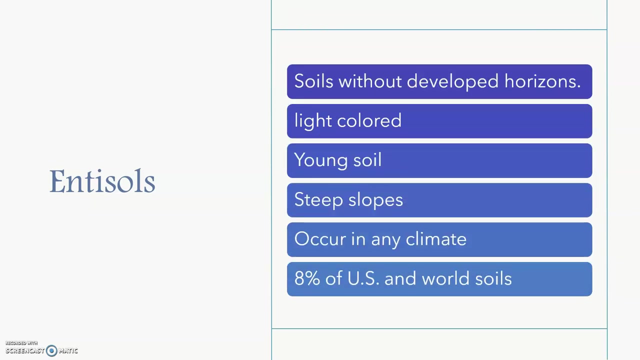 without dependence. Entosols are soils without dependence. Entosols are soils without developed horizons. You can't see the horizon very well in entosols. They are typically light-colored and are young soils. They have often developed on steep slopes and can occur in any climate. 8% of the United States and world soils are 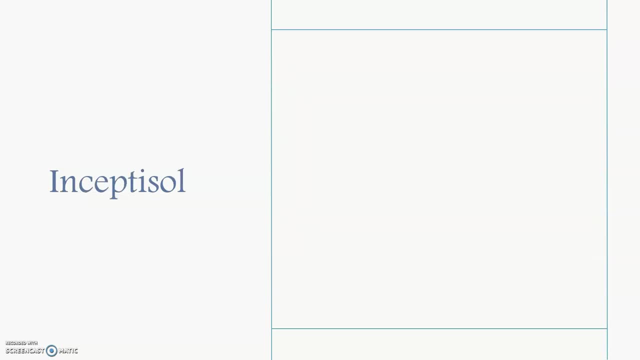 entosols. The next soil order being discussed is enceptosols. Enceptosols are weakly developed soils but are more developed than entosols. They are prone to erosion and tend to form on top of weathering rock. 18% of. 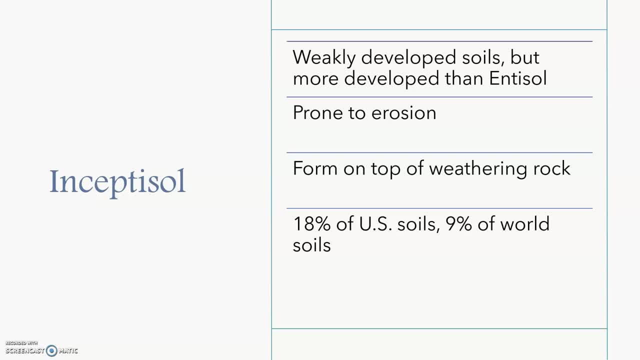 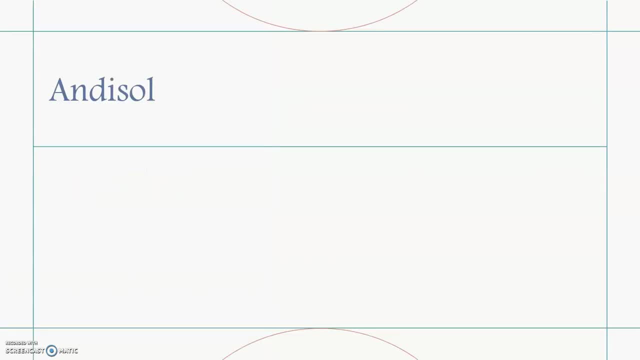 the United States soils and 9% of world soils are enceptosols. Enceptosols have a poorly developed surface horizon. Endosols are formed from volcanic ash. Endosols are dark, organic and fertile soils. They form in humid climates and in wet climates. Enceptosols are found in 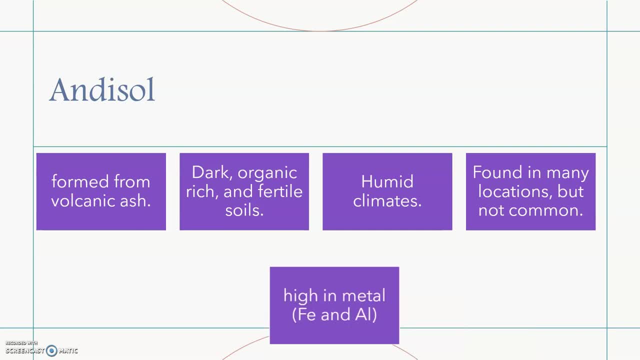 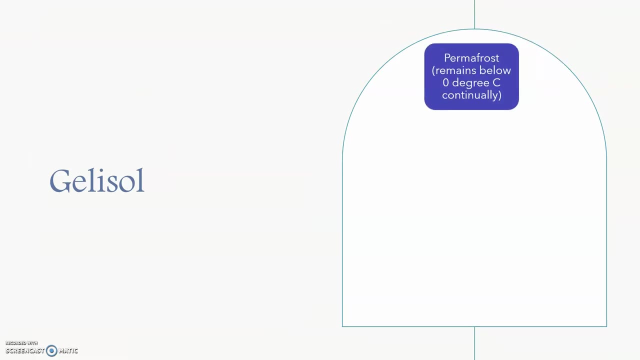 many locations but are not common. Andesols are high in metals, especially iron and aluminum. Andesols are typically young soils. Gelaceous are formed where permafrost is present. The permafrost is where the ground remains below zero degrees. 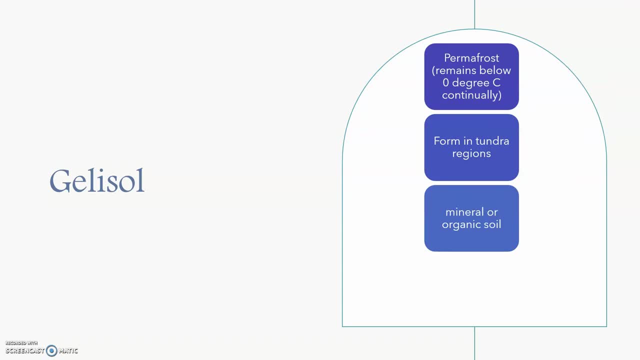 Gelaceous form in rondured regions, and Gelaceous can also form in mineral oxytocinarenamide. When Gelaceous are found, they packed from участes until they become dissolved in the Histosols. can be a mineral or organic soil. however, gelosols do show cryoturbation or 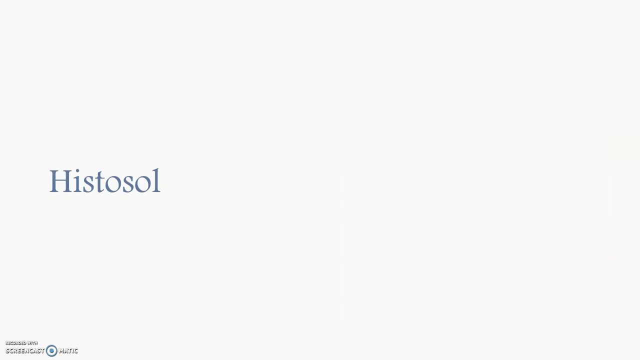 cold disturbance. The next soil being discussed is histosols. Histosols tend to be an organic soil and form under wet or cold conditions. Histosols have a spongy texture and are the least common soil order. Histosols tend to be dark in color and very lightweight when dry. however, they do have 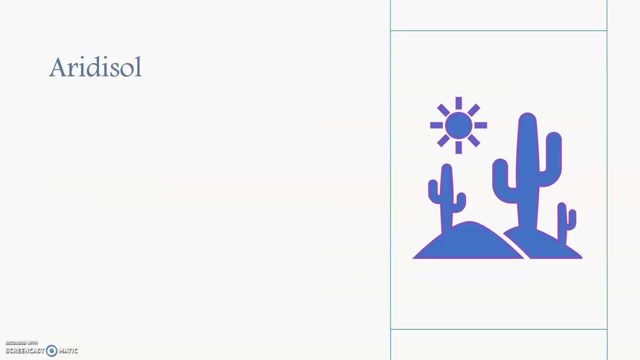 a very high water holding capacity. Next are aridosols. Aridosols are found in areas where it is dry for more than six months of the year, so typically deserts. There is an accumulation of calcium carbonate and salts. Aridosols are very productive when irrigated and are the second most common soil order. 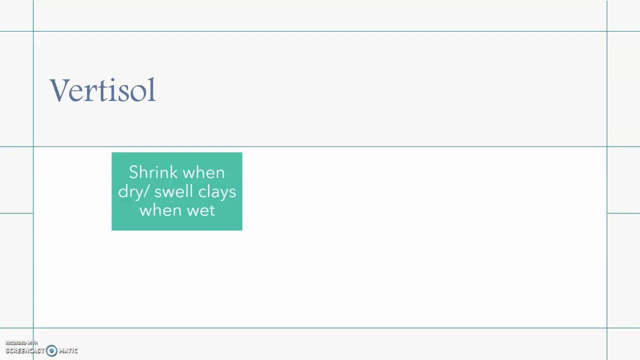 in the world. Next is vertosols. Vertosols shrink when dry and swell when wet. This is because there is a lot of clay. Vertosols have more than 30% clay. They are very fertile but are difficult to cultivate due to the clay content.